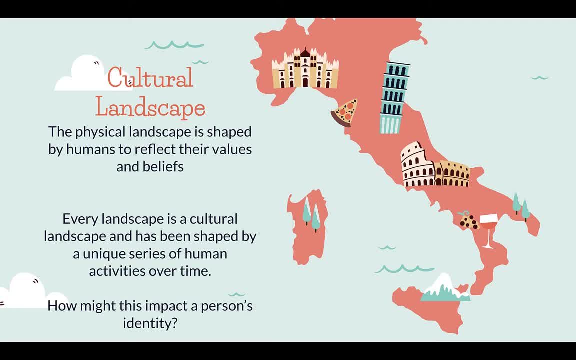 think about what's happened in each of those places that makes them so different. In Italy, we see a lot of things like the Catholic Church that really strongly impacts the cultural landscape, And in Greece we see Eastern Orthodoxy, because it's a lot closer to Turkey and Russia and has 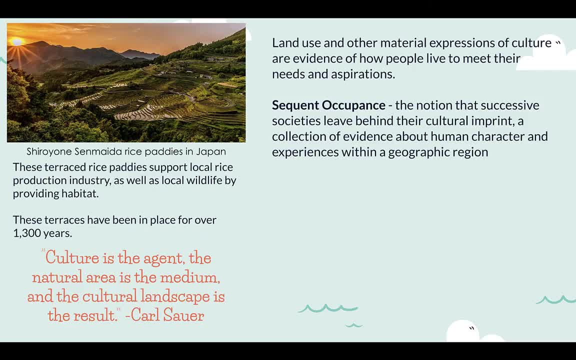 a lot of other influences that impact it. So the use and other material expressions of culture are evidence of how people live to meet their needs and aspirations. Basically, we change things to meet what we want and what we need. So, for example, we have the Shirayone Senmaida rice paddies in Japan And these are 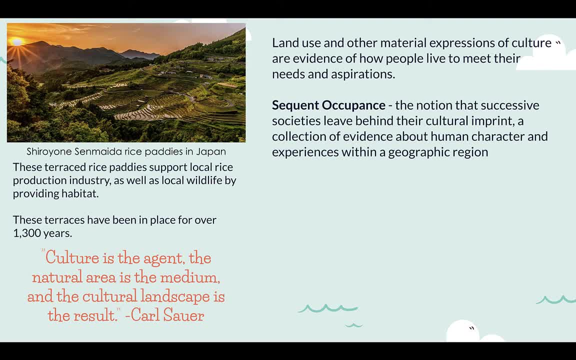 terraced rice paddies. They've been used for well over a thousand years, And not only do they support the local rice production industry, which is incredibly important, but they also provide habitats for local wildlife, Which is also important, because the natural landscape is incredibly important in Japan overall, but especially in this space. 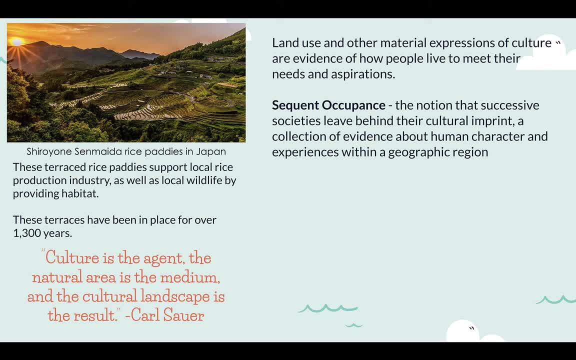 We also are looking at the idea of something called sequined occupants, or as in sequence, and then occupants, the people who are there. So this is the notion that successive societies leave behind their cultural imprint. It's a collection of evidence about human character and experiences within a geographic region. It basically says who was where and what did they do in that space, in their culture as well. So there's aaretHaidu's Honour and share funktioniert entre dans this to understand it within a geographic region market and have a saying of how they choose to choose, to choose. one. well, there's three things that objectively stand out, and we also have quite a lot in contrast there about movement and also central state schedule for personal waktu more so, but mainly comes to causal portal, Singapore's developement or growth. 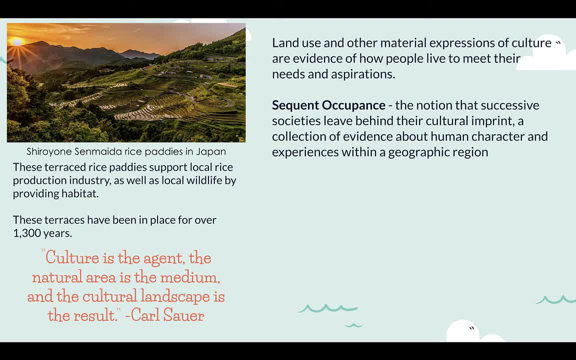 says who was where and what did they do in that space over a long period of time. So we have here a geographer by the name of Carl Sauer who saw landscapes as part of culture and as affected by culture, And he said that culture is the agent, the natural area is the medium and the cultural 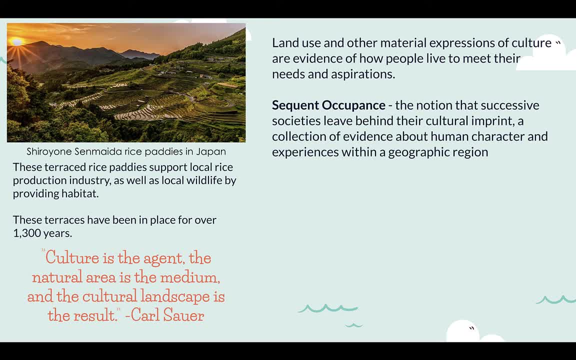 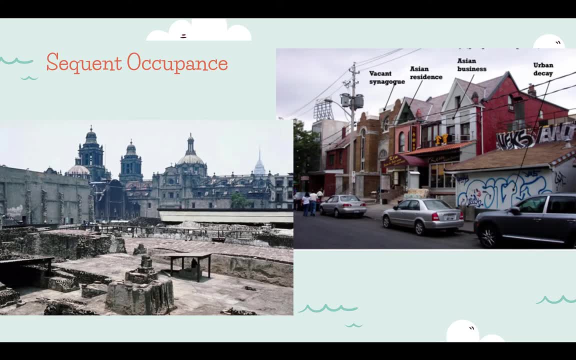 landscape is the result. So culture is what changes things, and what it changes is the natural area And ultimately, what we end up with is our cultural landscape. So, thinking about secret occupants, Here we have two different cities and we see the way that different generations have impacted this. 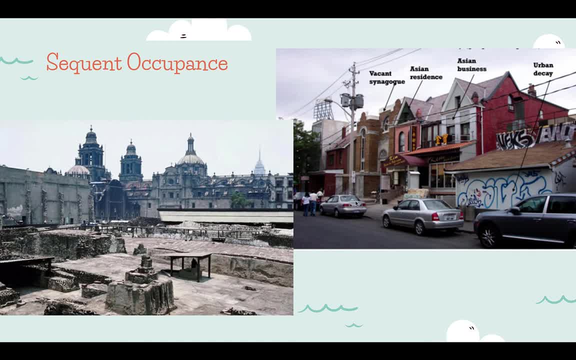 space On the left-hand side. so we have a vacant synagogue here, We have an Asian residence up here, We have an Asian business over here And here, where we see the graffiti and things breaking down, we have artifacts, urban decay. so we're seeing multiple generations of occupants on the right hand side. we're looking. 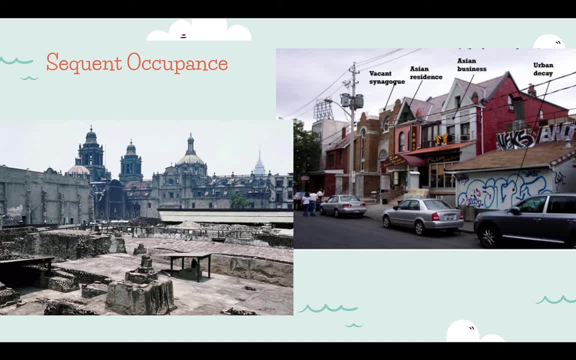 at mexico city and we can see once again multiple generations of occupants. in the foreground we have the templo mayor. so this is an ancient aztec temple or the remains of an agent ancient aztec temple. and the farther we get back, the newer the stuff. so we have a very large church or cathedral. 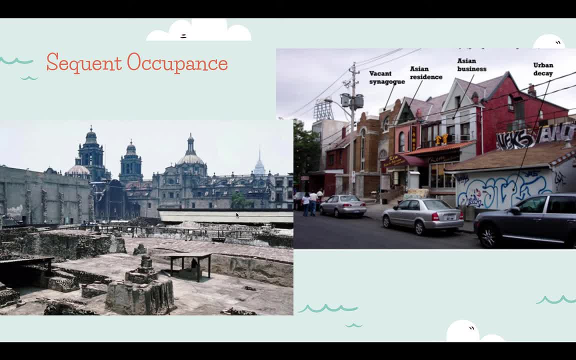 here, so that's going to reflect the spanish occupants. and even further on we start to see a skyscraper, so that's going to be even newer. we see multiple layers of civilizations in this one city and even in this one photograph. so looking at some examples of cultural landscape, 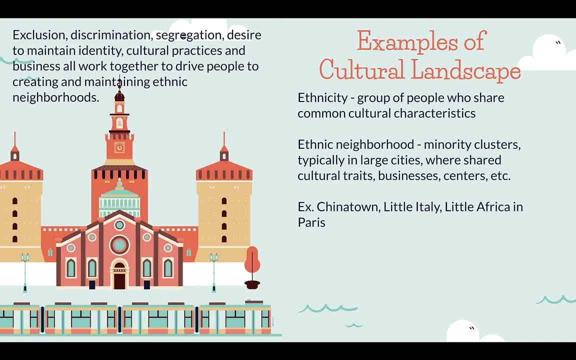 we want to think about things like ethnicity. ethnicity is really important and it refers to a group of people who share common cultural characteristics. ethnic neighborhoods pop up when we have minority groups who cluster, usually in large cities, so that they can share in their cultural traits, their businesses, their religious centers, their social centers, all kinds of things to get. 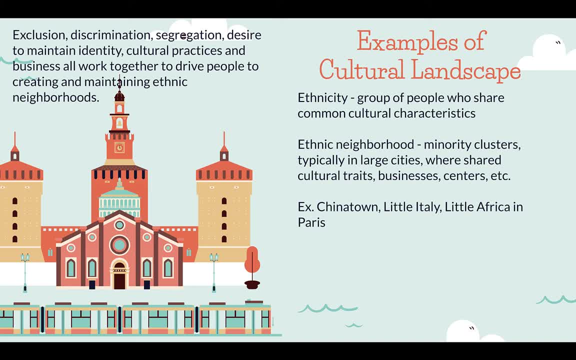 together, and some examples are chinatown, little italy and little africa in paris. these often pop up around things like exclusion, discrimination, segregation, overall the desire to maintain one's identity, to practice culture, to get into business or to go to businesses for buy people that are similar to you, that share. 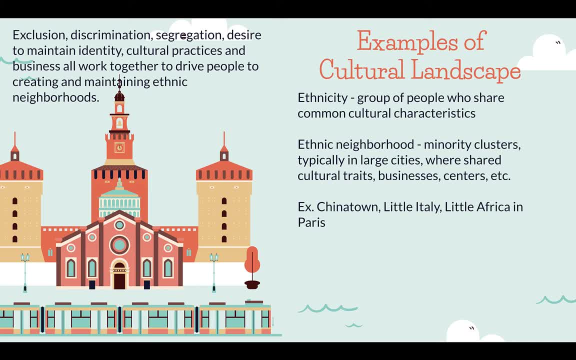 similar values that are selling stuff that you're familiar with. essentially, people are driven to put all of this stuff together to create and maintain these ethnic neighborhoods. they want to be with people who are like them, and so we see these different ethnic neighborhoods where we see larger collections of particular groups of people who exist within these neighborhoods and 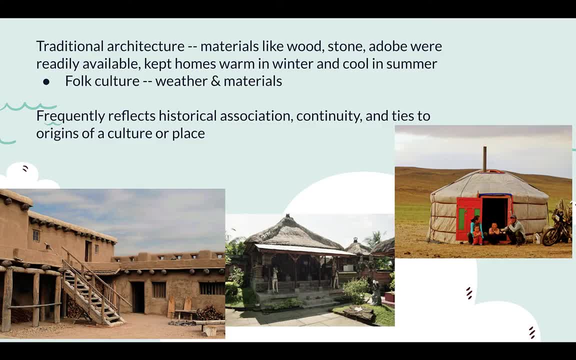 they also see the most similar cultures within the larger cultural landscape. looking at traditional architecture- so this is largely what we think of as folk architecture- we start to see materials like wood, stone and adobe being used. this is because they're readily available and they often serve the 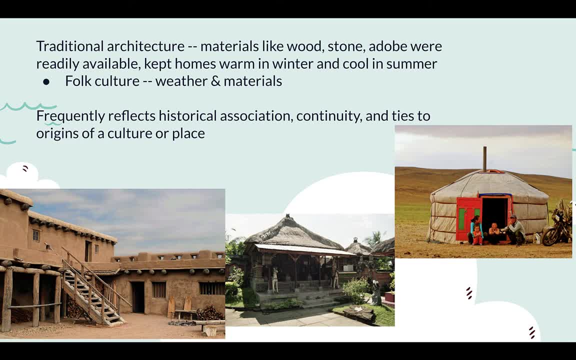 purpose really well. so they keep homes very warm in the winter and they keep them cool in the summer, when we don't have access to things like air conditioning or electric heat. basically, folk culture depends on weather. folk architecture depends on weather and materials. It also is going to frequently reflect historical association, continuity and ties to the origins. 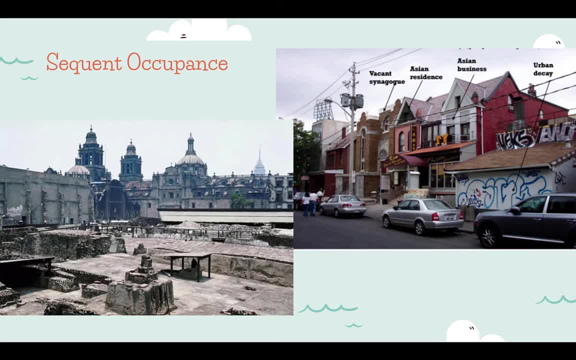 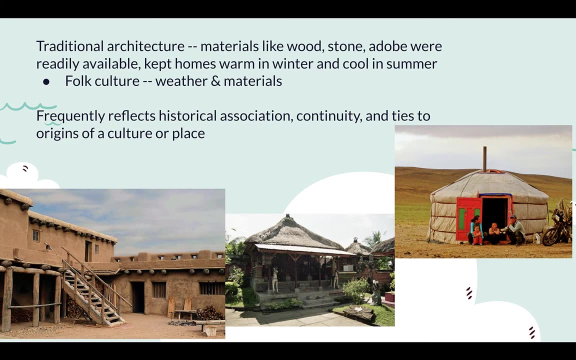 of a culture or place. So, going back to this picture in Mexico City, where we see the Aztecs here and then the Spanish invaders here, and each brings a particular piece to that history, to that story, Here we're looking at an adobo home. 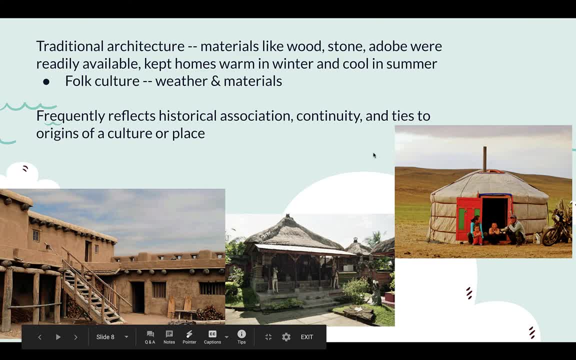 Here we're looking at wood with a thatch roof and here is something called a gur, and this is in Mongolia. Many ethnic Mongolians are nomadic even today, and have been historically So. they have homes that are essentially very structured, They're tents, and they provide a significant shelter when it's colder or when you are stopped. 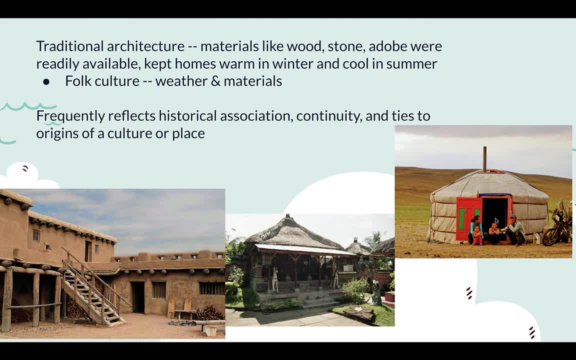 You can see. it has a chimney coming out the middle. There is going to be a stove in here, but it also is packable so that when you leave a place you take your home with you. And this one here is kind of an interesting combination of folk and popular culture, because 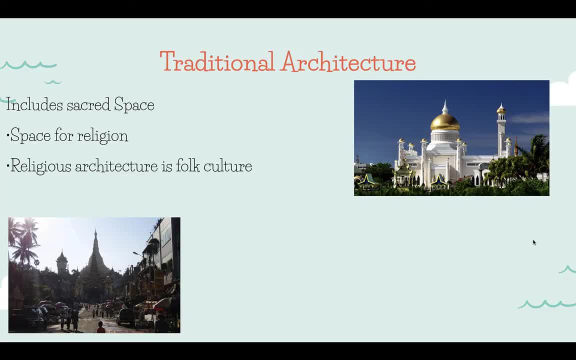 we can see the gur in the middle, but we see the motorbike on the side. With the traditional architecture, we also include sacred spaces. So this is space for worship, This is space for religion, space for spiritual practice, whatever it happens to be. 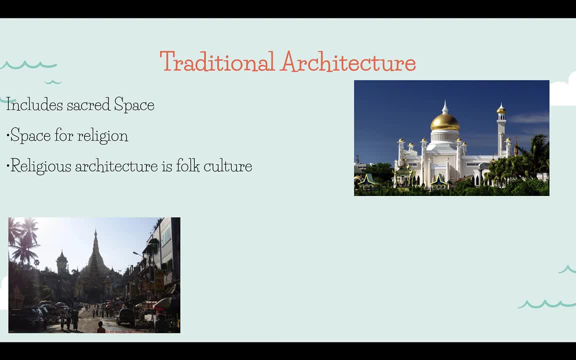 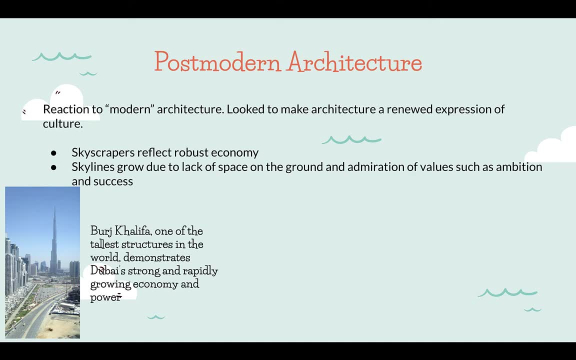 And religious architecture is considered folk architecture, whether it's what we would consider a popular or major religion or not. Then we move on to postmodern architecture. So back in the 50s and 60s we have a lot of new architecture popping up, stuff that. 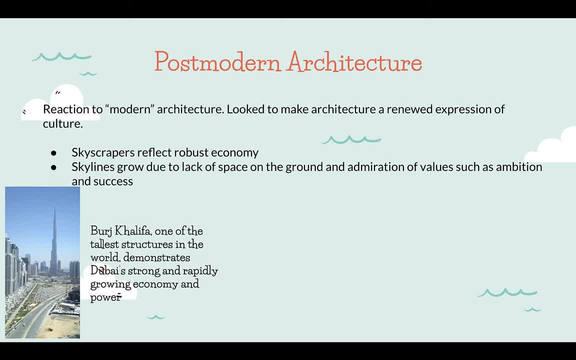 we don't consider to be very pretty or aesthetically pleasing by modern standards, And so postmodern architecture kind of pops up as an answer to that. They look to make architecture a renewed expression of culture. So once upon a time it had been, and then it really didn't feel like it was anymore. 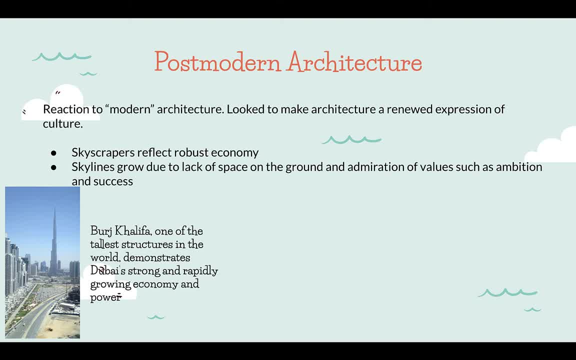 So they changed architectural styles to once again reflect culture. So with this we get a lot of things like skyscrapers, And skyscrapers are going to reflect a very robust economy. They're expensive, They're difficult to build, They need a lot of engineering and safety. 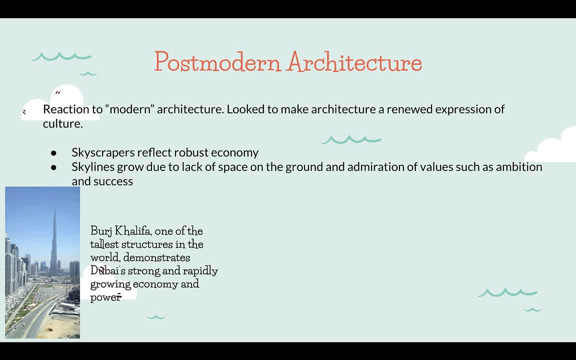 So having a strong economy is going to mean that your cities have more skyscrapers. This also has other implications. There are fewer skyscrapers where we have a lot of earthquakes or where we have a lot of windy storms like hurricanes. Florida, for example, doesn't have a lot of very tall skyscrapers because a lot of hurricanes 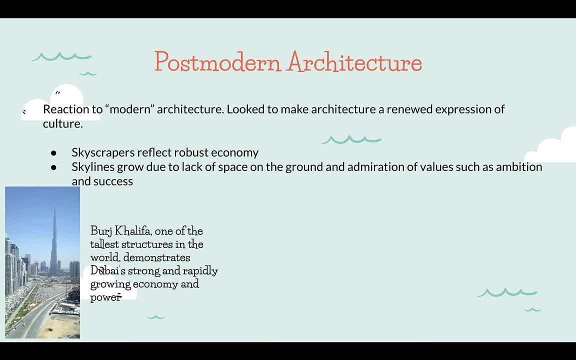 blow through and it's not safe. Therefore, we tend to have much more sprawling buildings, But cities like New York, where we don't have earthquakes- Earthquakes basically ever- or hurricanes- Buildings are much taller Spaces at a premium And this kind of hits on that next one where we have not a whole lot of ground space but 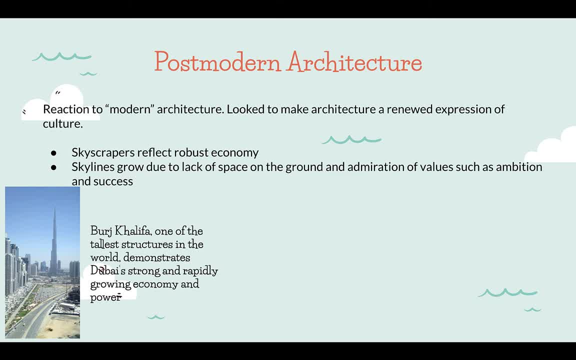 we look to increase our utility of a space, So we go up, So skylines grow due to a lack of space on the ground and by admiration of values such as ambition and success. Yeah, Yeah, It's a skyscraper. that's ambitious. 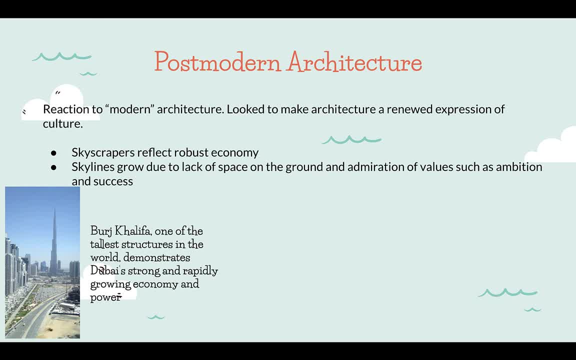 So it is defying the laws of gravity- gravity- But it's also a show of success. It's a show of economic success, engineering success, overall, things that we value in American culture in particular, but in Western culture as a whole. 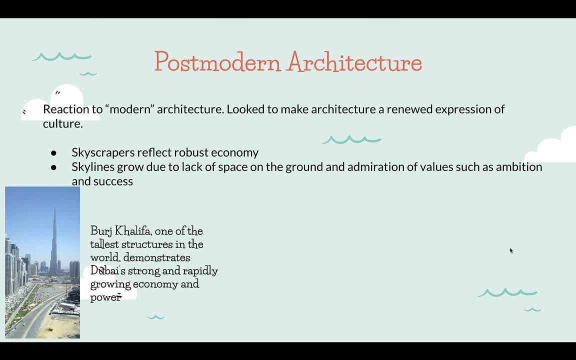 So one of the tallest buildings in the world, the Burj Khalifa, is in Dubai And this demonstrates Dubai's very strong and rapidly growing economy and power. And it's not just a country, It's a country, And you can see when you look here. this is much, much taller than any of the other buildings.